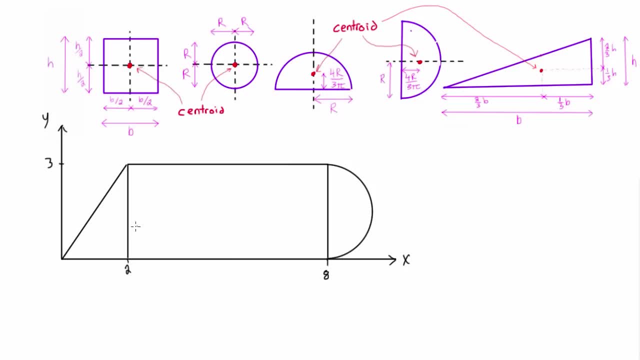 shapes, that we already know where the centroids are And then we add them up together, sort of using that discrete method that I was talking about in one of the last and I think in the last video, where we to find the centroid of multiple things, we have just the sum of xi times the area. 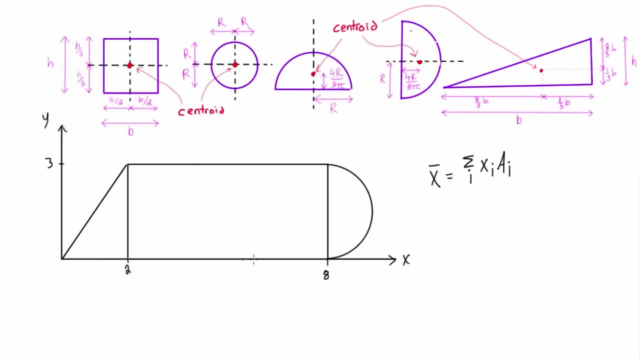 So that would be the centroid along the x component of the centroid and the area of that individual shape And that was over just the total area of the thing that we're looking at. So we're going to be using this formula And basically we just know that the 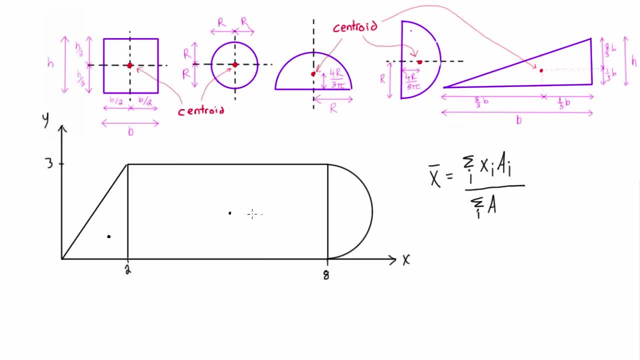 centroid for the triangle is going to be somewhere like that. The centroid of the square will be somewhere in the middle, will be in the middle, And the centroid of this semicircle will be according to this formula. So what we want to do here is we want to get each component here, So the 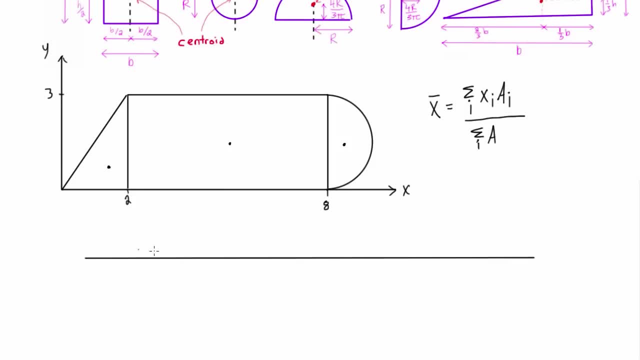 first thing we're going to do is we're going to construct a bit of a table here. So let's go like this. We'll do it sort of by parts, So we'll have first of all, we'll have the triangle, and then we'll do. 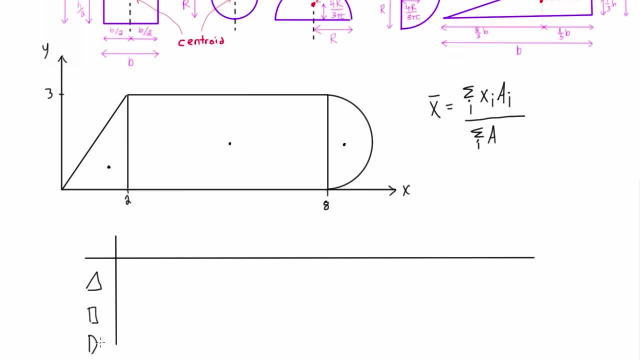 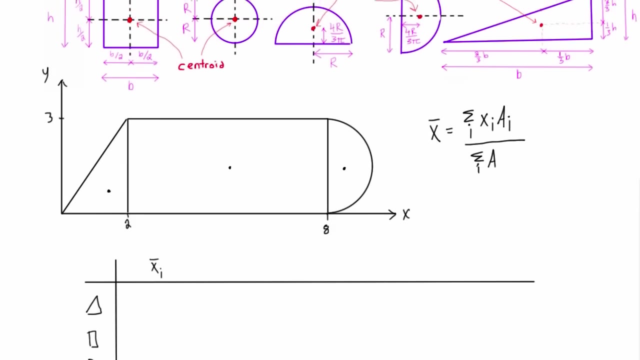 the stuff for the square and then lastly, the semicircle. So the first thing that we need to calculate for each individual shape is the component, the x component, of its own little centroid here. So to calculate the centroid of a triangle, basically we need to be 2, 3rds away from the short side, and that's going to give us the x component. 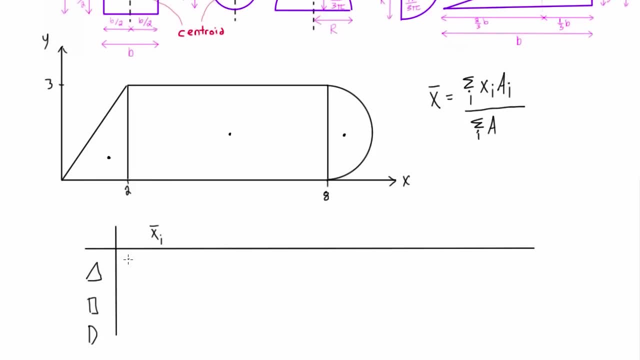 So that's simply just 2 3rds times the base, And in this case the base is 2, so we have 2 times 2 over 3.. And that's also just going to give us 4 3rds. So that is the x component of the. 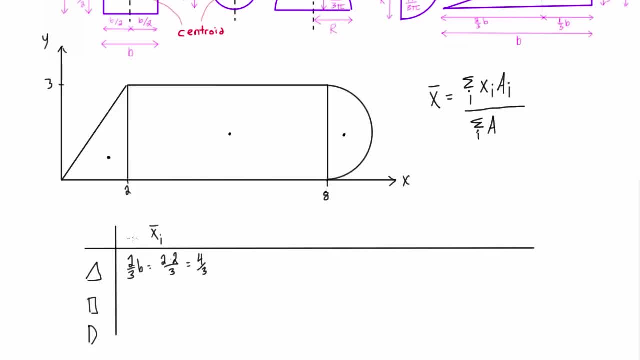 centroid here or the centroid along the x axis For the square, it'll be halfway along the base. So the base is 8 minus 2, so it's 6 units long. But we also have to add in this 2 here, because 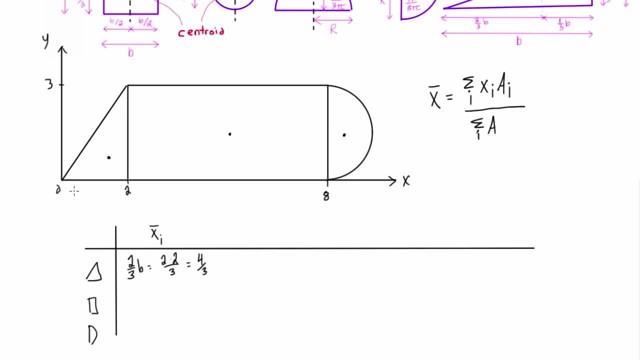 it's from the 0 here that we're looking at. So it's going to be 2 plus 1 half base, And this is the base of the square. in this case, 2 plus, well, 1 half. The base was 8 minus 2, which is 6.. 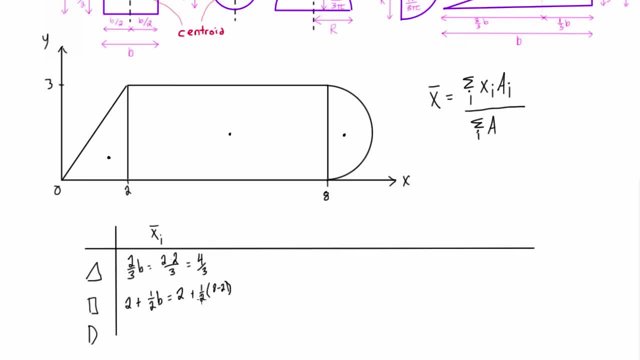 So we have 6 divided by 2 is 3, plus 2, that gives us 5.. So we can even draw these on. Maybe let's change the color here. So this x bar here is located at 4 3rds. 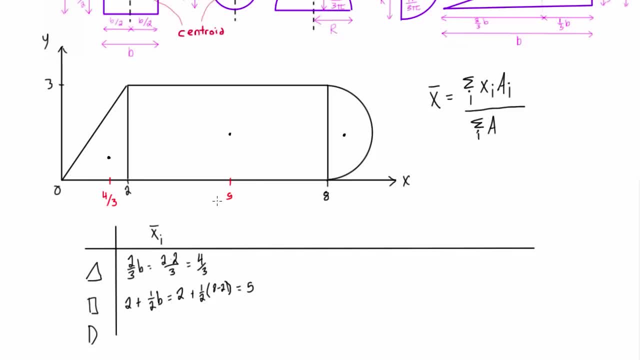 This one here. its location on the x axis is 5.. And then, if we go and figure out the last one here for the x location of this, well, we have to first we know that the x, we can find the centroid using this little formula. 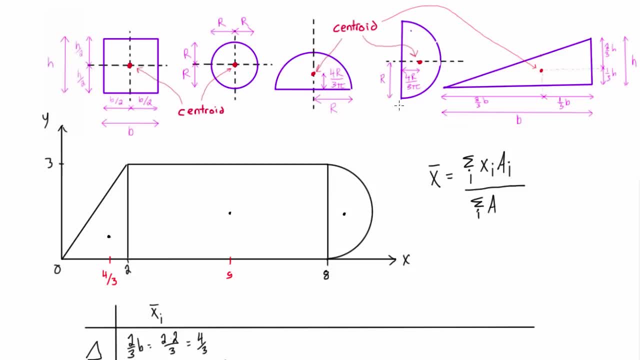 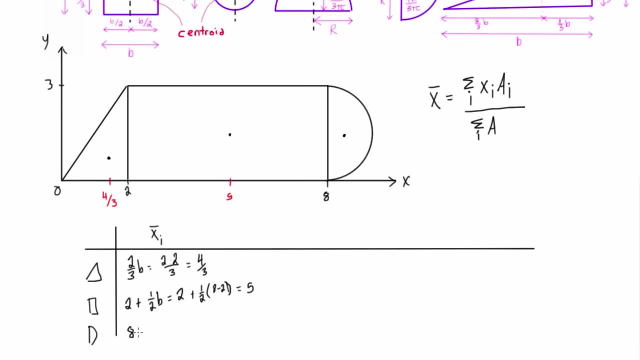 here based on where the start of the semicircle is. But the semicircle is also 8 units away from the origin, So we just got to start off by adding in 8 plus, and the formula is up here: It is 4. 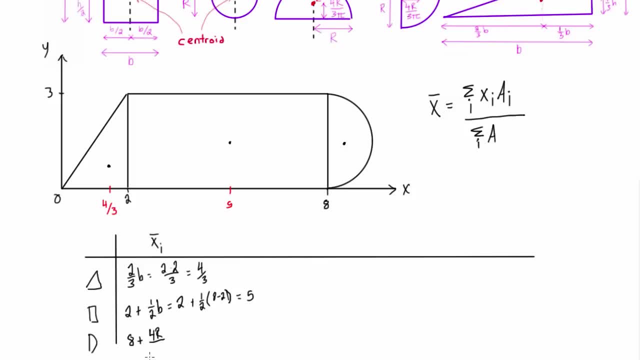 times r over 3 pi And the radius here. you can pick this off the diagram. Sometimes it won't be given to you, but clearly if this is 3 units tall and this is half of a circle, then the radius here is going to be: 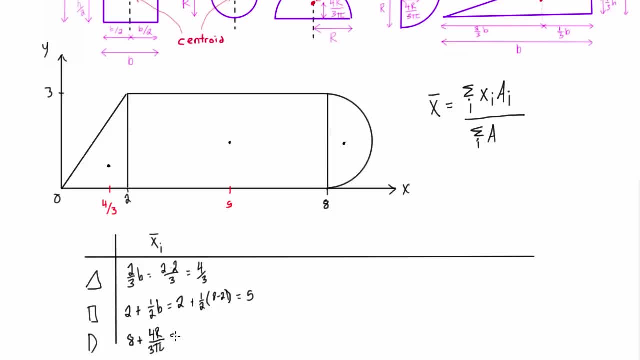 half of that height. So the radius is going to be 1.5.. So we get 8 plus 4 times the radius, which is 1.5, over 3 times pi, And if you just solve that, this term here is going to be about 0.64 and add it. 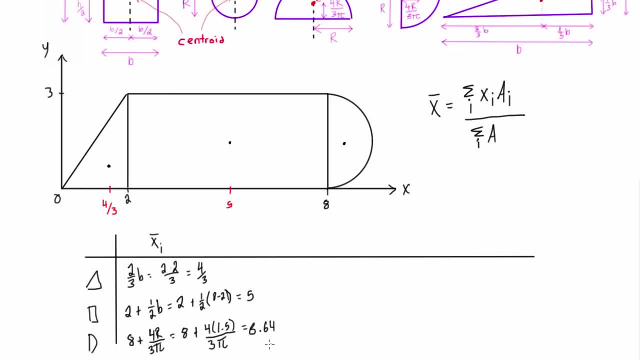 to 8, so we get 8.64.. Alright, so we've got all of the xi, the, the- what do you call those things? the centroids, the location of the centroid on the x axis. There we go: 8.64 for that guy. Alright. so the next thing we need: 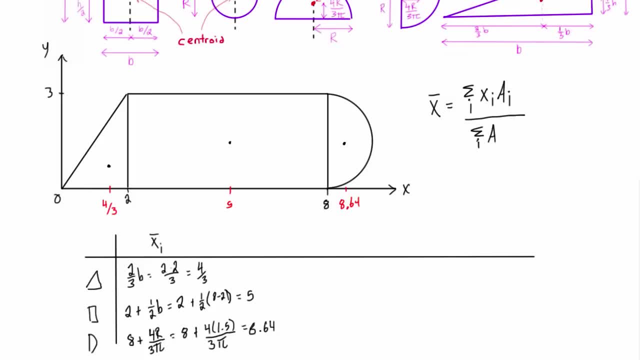 to do is we just need to figure out what the areas are for each of these compound shapes. So let's put in the next part of our table here And we'll do each individual area, And this is pretty easy. The area of a triangle is just 1.5 base height. 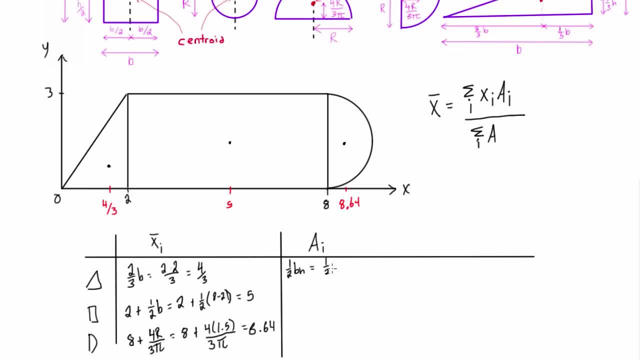 1.5 times base times height, And in this case our base is 2, and our height is 3.. So that's going to give us an area of just 3 units there, Area of a square, simply base times height. We figured out our. 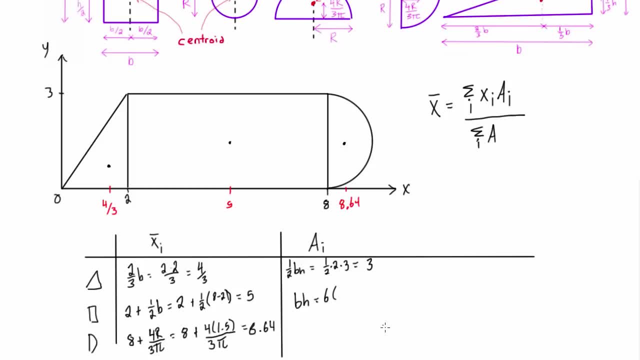 base here was 6 units, and our height here is 3 units, So that just gives us 18.. And then for the area of a semicircle, that's just well. the area of a circle is pi? r squared, so 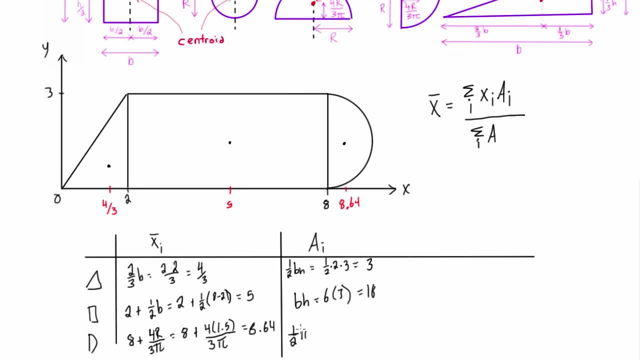 this is just half of that, So 1.5 pi r squared, And we know what all these numbers are. so that's 1.5 pi and our radius was 1.5 squared. Alright, and if we just calculate that, we get that's. 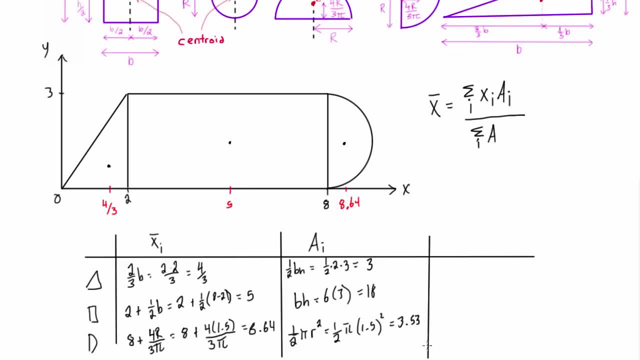 3.53.. Okay, cool, Moving on, What we want to do now is just to simplify our life here for this equation. we can do this. we can multiply these two bits here in the table itself, So we'll just put in: 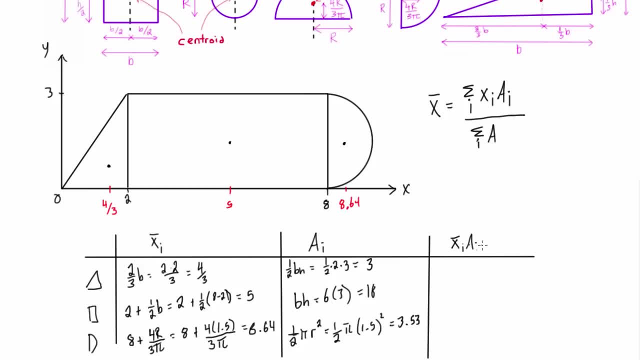 a column here. so xi times ai times ai, and so we have xi, 4 thirds times ai, 3.. So for the triangle, 4 thirds times 3, that's just going to give us 4 units. And you'll see, we could do this all in the equation, but it's just a little bit easier to organize. 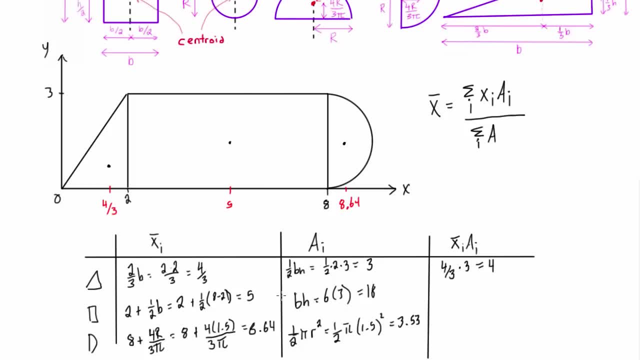 it here in the table. So for the square, it's xi is 5 times 18, which is that? so 5 times 18, that's going to give us a value of 90.. And then lastly down here, so we just have 8.64.